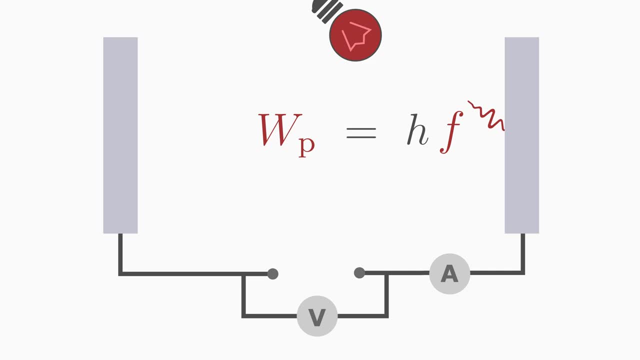 then nothing happens. But if the energy of the photon is high enough, then the photon knocks an electron out of the plate. The energy necessary to eject an electron is called the work function W Only when the photon has an energy greater than the work. 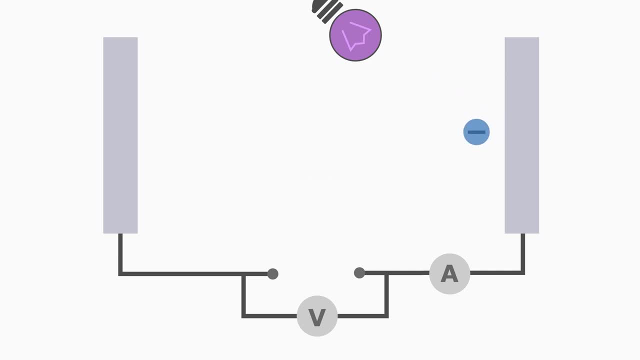 function energy, then it can knock out an electron out of the plate. You can determine the work function easily because you know how to determine the photon energy. If you increase the light frequency, you will eventually arrive at a photon energy that is sufficient to eject an electron. This light frequency used, above which the electron. 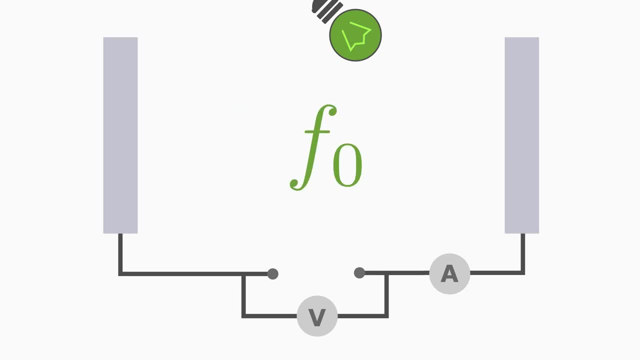 is ejected is called the threshold frequency F0. Sometimes it is called a cut-off frequency. If you multiply it with the Planck's constant, then you get the required energy of a photon. You get the work function W. As I said before, if you don't know the frequency, 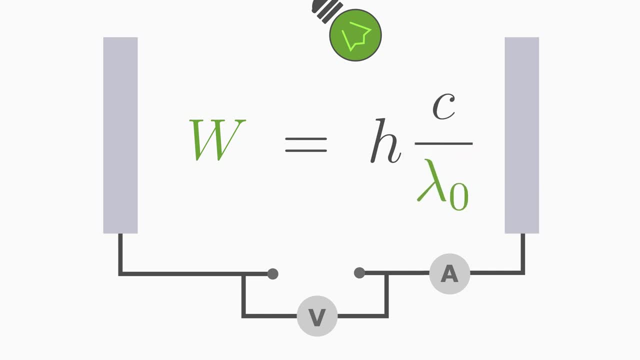 but the wavelength. then you can also calculate the work function with h times C divided by lambda0.. Here lambda0 is the threshold or cut-off wavelength. The work function depends of course on the material used for the electrode, For example: 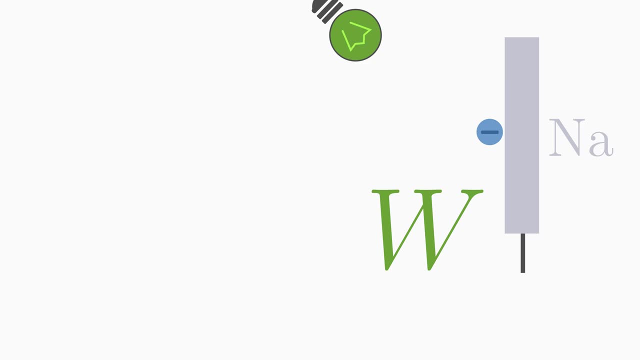 For example, it is easier to knock out an electron from a natrium plate than from an aluminium plate. For a natrium plate, the photon must have at least 3.6 times 10 to the power of minus 19 joules. 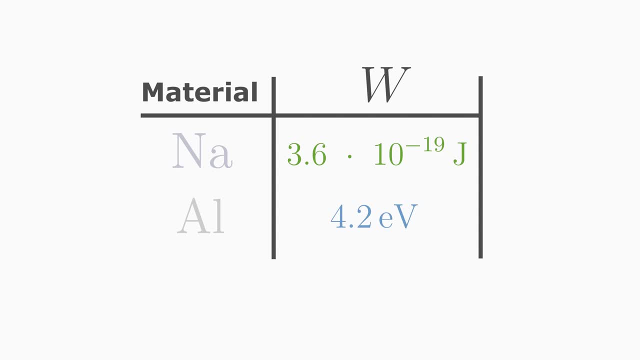 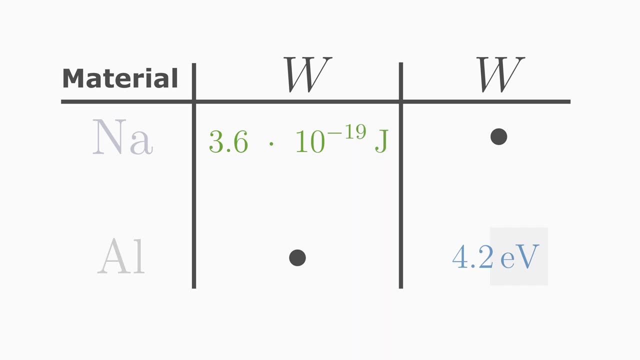 For an aluminium electrode the photon must have at least 4.2 electron volts. I use different units to show that energy is often expressed in electron volts. You can easily convert joules into electron volts and vice versa. If the energy is given in joules, then divide it by the value of the elementary charge: 1.6. 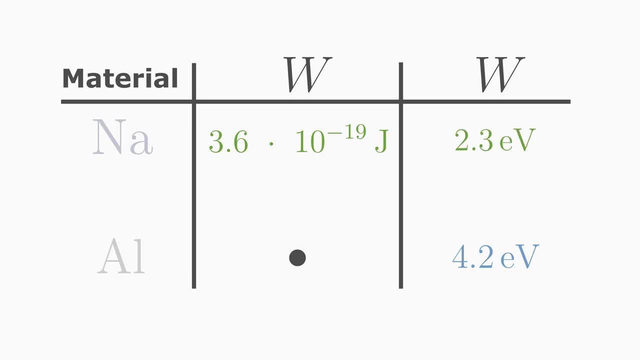 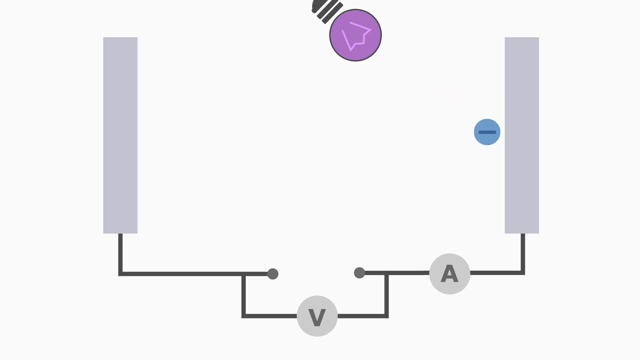 times 10 to the power of minus 19 to get the value in electron volts. If the energy is in electron volts, then multiply it by the value of the elementary charge to convert it into joules. After a photon has overcome the work function of the plate, and the energy is given in joules, then divide it by the value of the elementary charge to convert it into joules. after a photon has overcome the work function of the plate and the energy is given in joules, then divide it by the value of the elementary charge to convert it into joules. 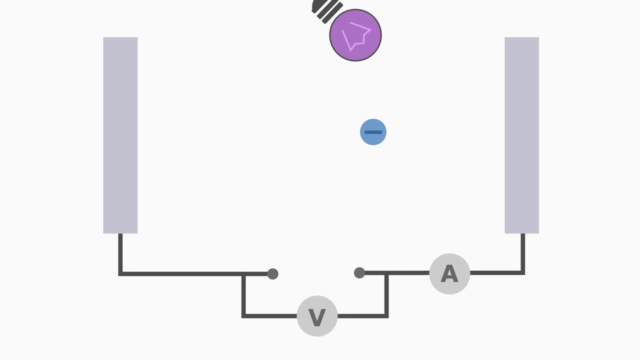 After a photon has overcome the work function of the plate and knocked out an electron, the electron leaves the plate with a certain velocity V. The electron leaves the plate with a certain velocity V. So the electron has a kinetic energy. let's call it W-kin. 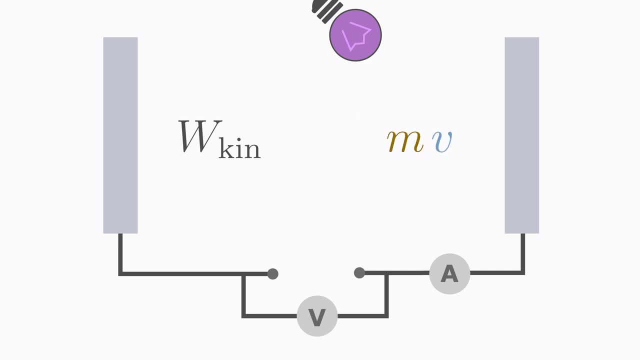 If we know the velocity of the electron, we can calculate it quite easily, namely with 1.5mV-squared. we can calculate it quite easily, namely with 1.5mV-squared. The mass of the electron has the value 9.1 times 10, to the power of minus 31 kilogram. 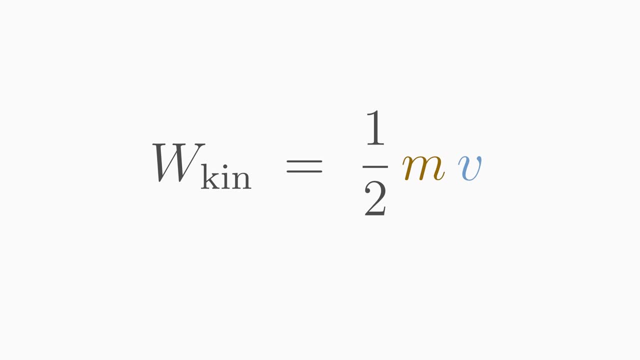 But where does this energy come from? It cannot have been created for any other reason: been created out of nothing. Let's look at the conservation of energy. We have used the energy of a photon. Only this energy is available to us. A part of it was used to overcome the work function. 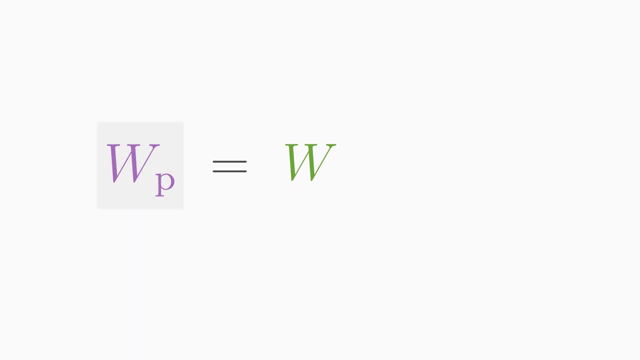 And what if the photon had a larger energy than the work function? Where did this remaining energy go? Exactly, this remaining energy is the kinetic energy of the electron. So, according to the conservation of energy, we have derived a formula for the photoelectric effect. 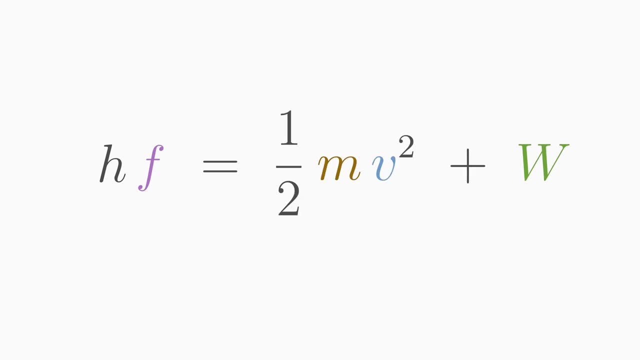 Photon energy equals kinetic energy plus work function. This is the so-called Einstein formula for the photoelectric effect. How do we even know that an electron is moving out of the plate at some velocity? Of course we can't see it with our naked eyes. This is where the plate capacitor 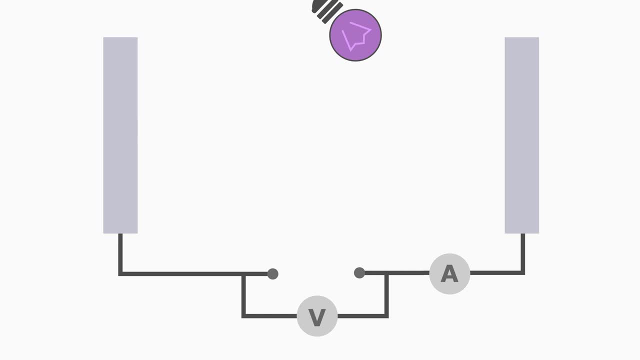 comes in, We switch on the plate capacitor in such a way that the plate which is irradiated with light is positively charged and the opposite plate is negatively charged. As a result, ejected electrons are slowed down because they are repelled by the opposite plate. We can increase this repulsion by increasing the voltage between. 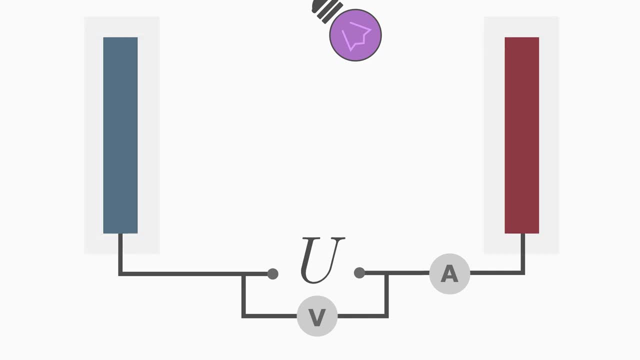 the plates. When we set the polarity of the capacitor in such a way so that the electrons are slowed down, we call the voltage as breaking or stopping voltage. If the voltage is not large enough, then our ammeter will show some non-zero value. 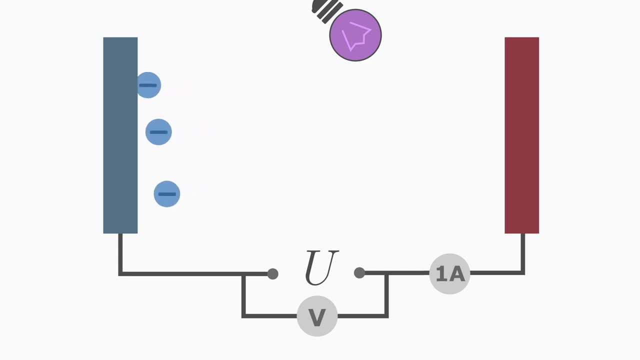 because electrons are able to reach the opposite plate. But when we set a voltage value- let's call it U0, at which the current has dropped to zero, then no electron arrives at the opposite plate. This value of the voltage at which the current